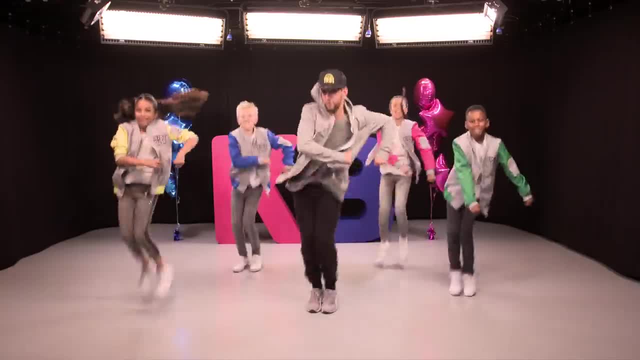 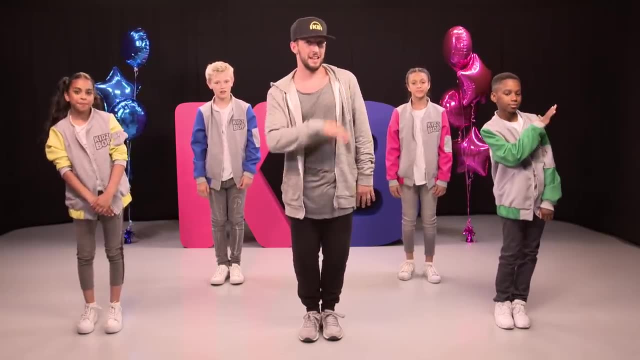 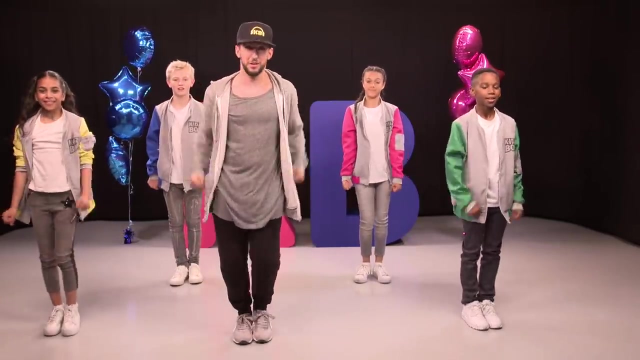 six, seven, go one, two, three, four, brush, brush, brush, brush. very good, now these are on the dance, dance, dance, dance. now, from here you're stepping out with your right foot, you're gonna go double pump, pump, pump together, single pump, single pump together. we repeat our little dance, dance, dance. 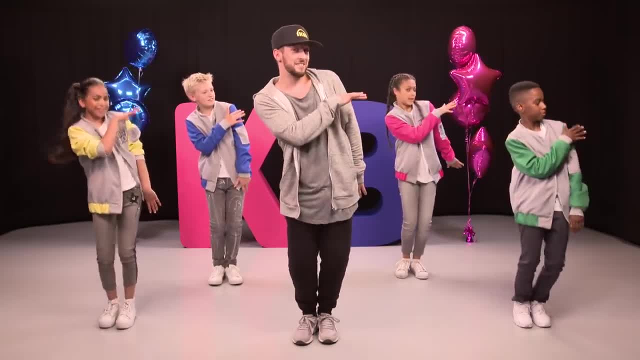 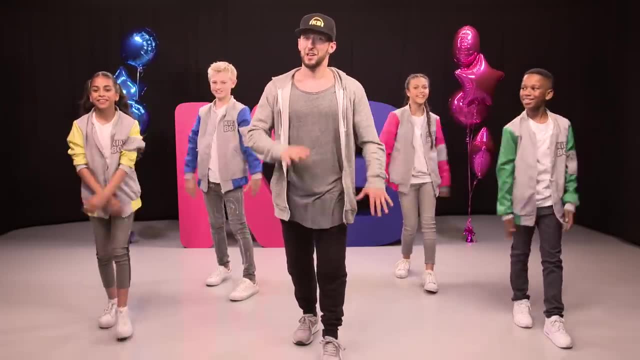 dance move and you're gonna go dance, dance, dance. now, this time you only do one on the left shoulder, left shoulder, and you're gonna step forward your left foot. come on now. that can be whatever you want, but he says in the music: come on. and it's like you saying: come on, mom and dad, join me dance. 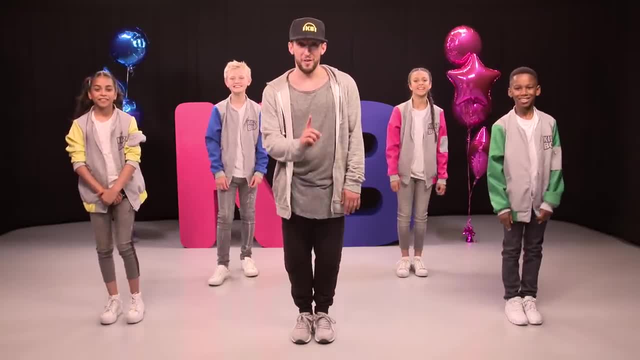 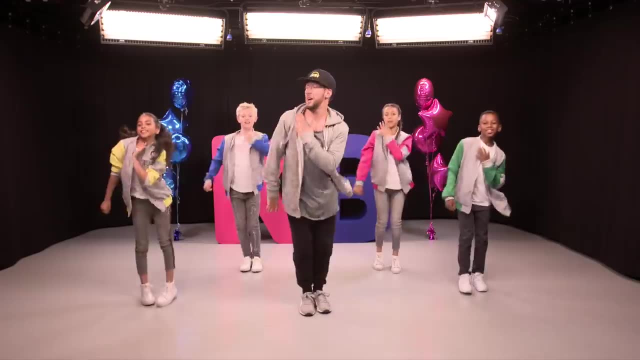 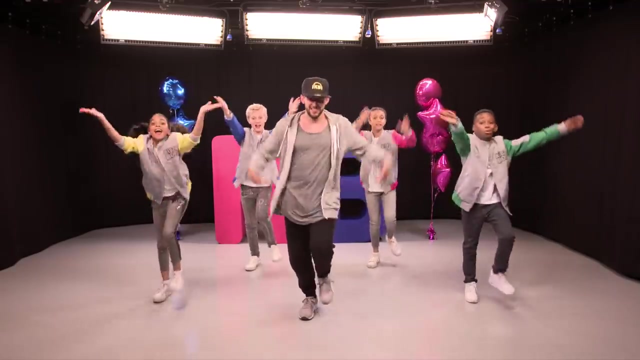 well, they can. if they want, let's go from the very top, add the whole thing together. okay, here we go. five, six, seven, go jump. two, three, four, dance dance double pump. one and two, three, four, dance, dance dance. come on, very, very good, lovely, from here we're going to carry straight on. you step with. 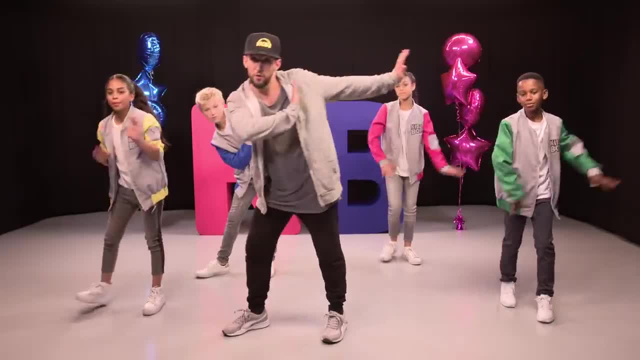 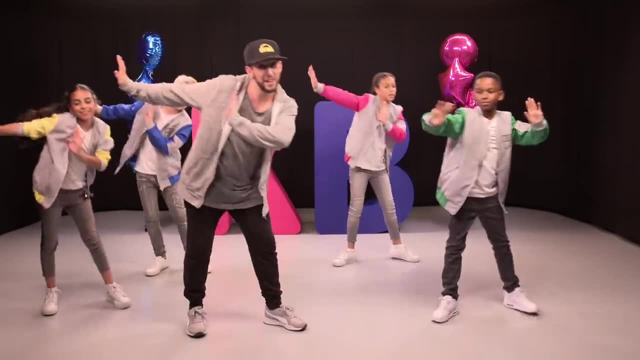 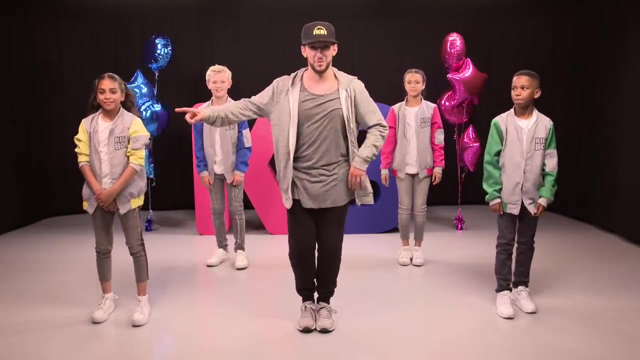 your right foot towards your right and you're gonna go: flick the hands, come in, flick the hands, come in. you do the same step going towards your left. flick the hands, come in, flick the hands, come in. now this step is actually called the janet jackson. let's practice the janet jackson here. 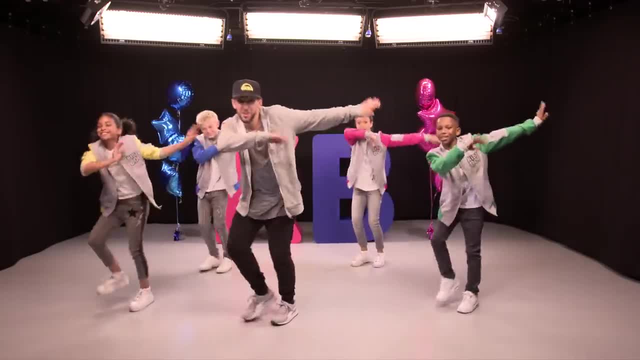 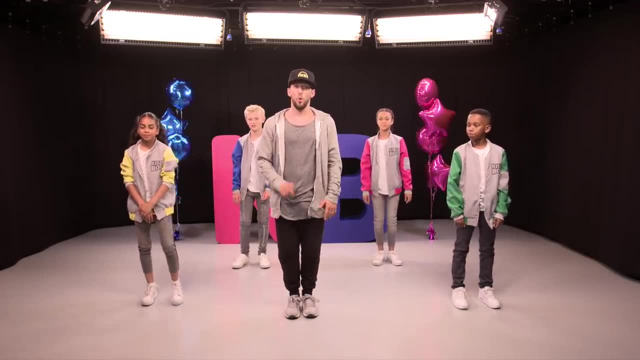 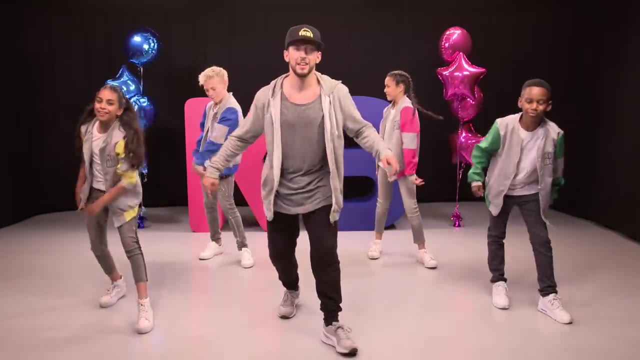 we go five, six, seven, go one and two, three and four, five and six, seven and eight. very, very good, we're gonna carry on just a little bit more. one step from here you're gonna do box step. you'll start with your right foot going forward. you're gonna go out out, in, in, out, out, in, in simple. 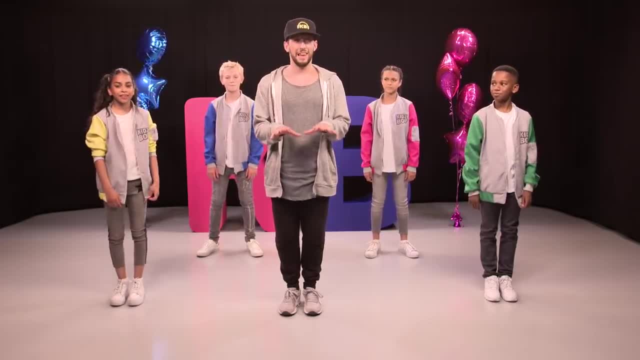 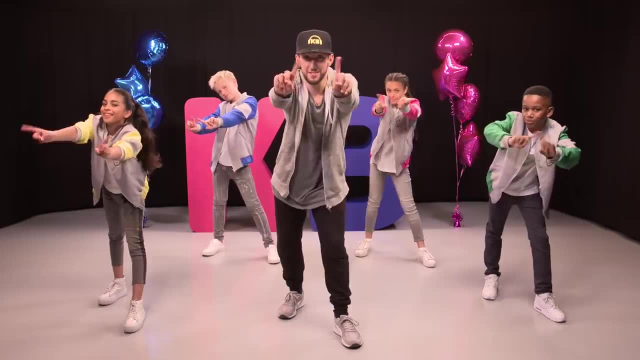 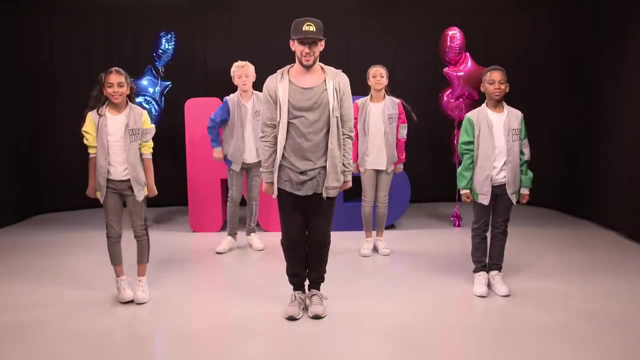 box step. if that's okay with you, you can stay with that. if you want something a little bit more challenging, you're going to add the arms on top. you're going to go out with the arms. out. the arms wiggle, the fingers wiggle, the fingers roll, the arms roll, the arms roll and down. now the lyrics. 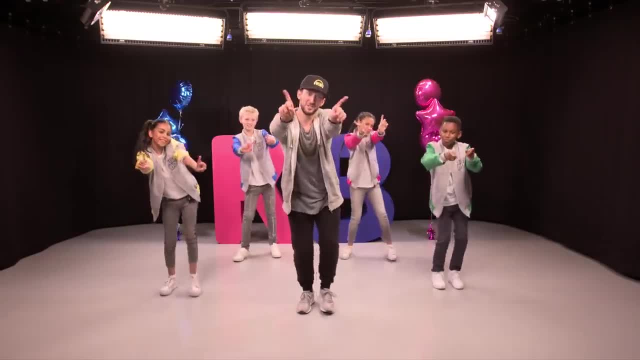 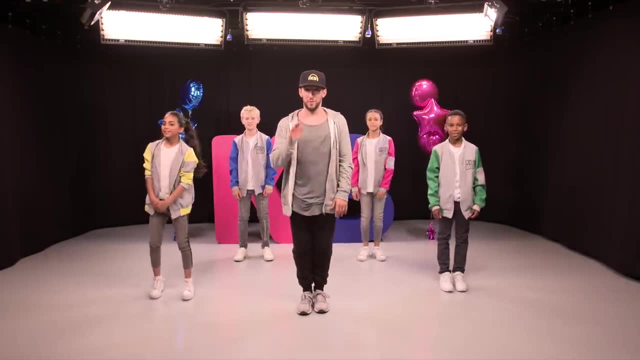 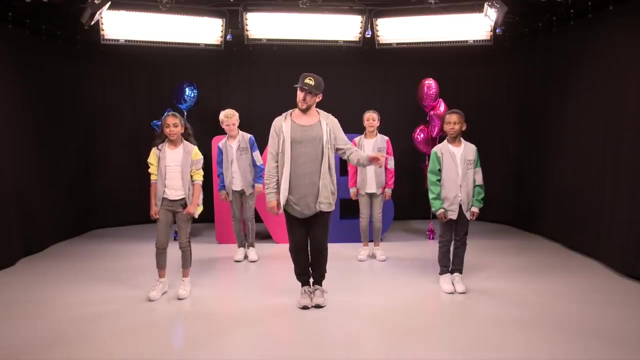 he says: Nobody leaving, so just keep dancing. six, seven. So it goes with the lyrics and the moves together. Okay, let's go from the very, very top slowly, Is that cool you? yeah, You're ready to go slow. Yes, here We go from the top ready, jump into your left first. five, six, seven, go one. 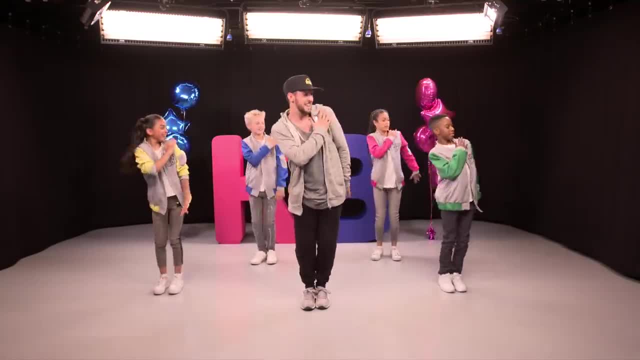 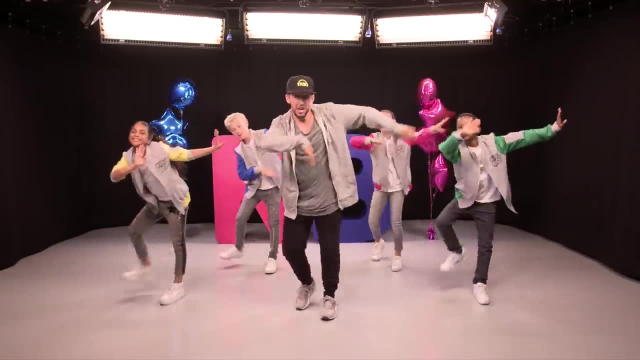 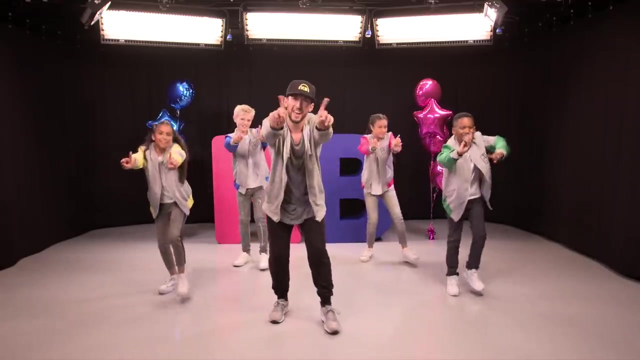 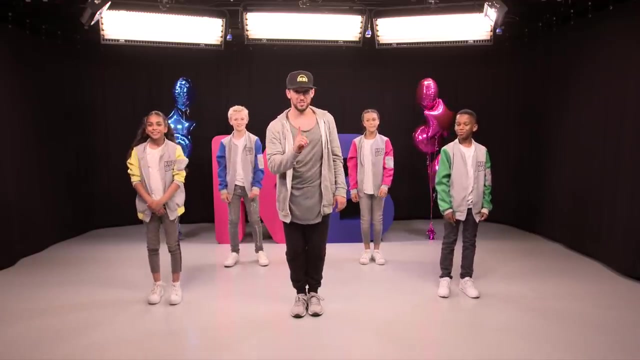 two, three, four, Dance, dance, dance, dance, good, good creeping up on you, So just dance, dance, dance. come on, Janet Jackson, Janet Jackson, Hey, Hey box. step one and two, three and four, roll, six, seven, eight. You're doing great guys, Really really good from here. We've got one more step two. I lied. 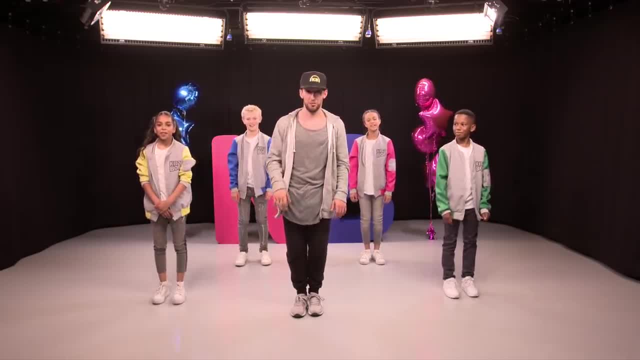 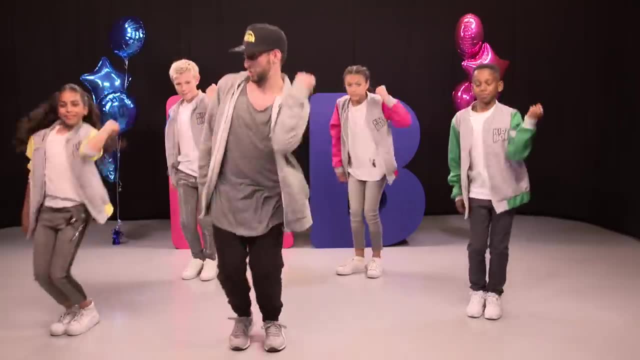 You're gonna go jump into the right twice. This step is called the Reebok. You're gonna grab your left fist like this two little bunny hops while you push forward. You're gonna go push, Push other side, push, push. now, from here you slide to your right, slide, put the foot behind. 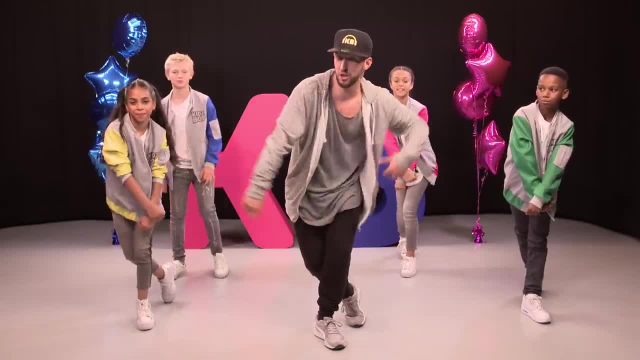 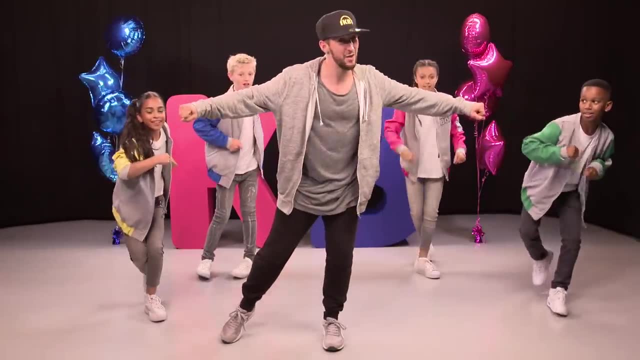 Slide, put the foot behind. you repeat that step again from the Reebok. You're gonna go one, two, three, four, slide, five, six, Seven, and now from here you repeat your come on, but you step back in your right foot, come on, And you can do whatever you want to do. 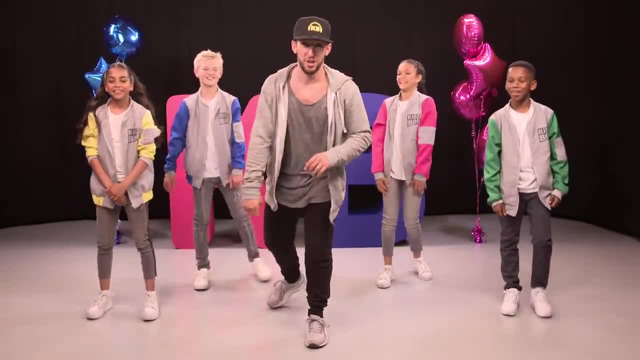 Everyone has their own sort of style. You can pick your own style. Okay, so that last step is simply Reebok, Reebok, Reebok, Reebok, slide, slide, slide, Come on. Okay, we're gonna do from the Reebok slowly. 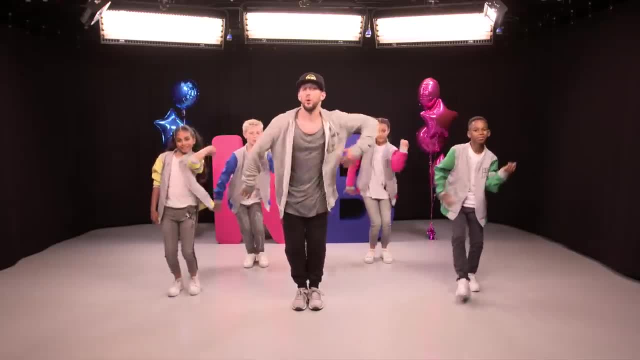 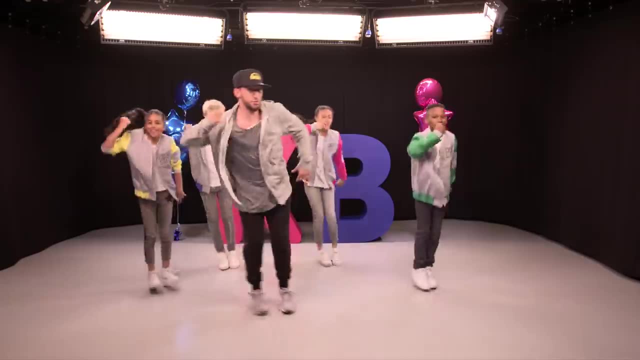 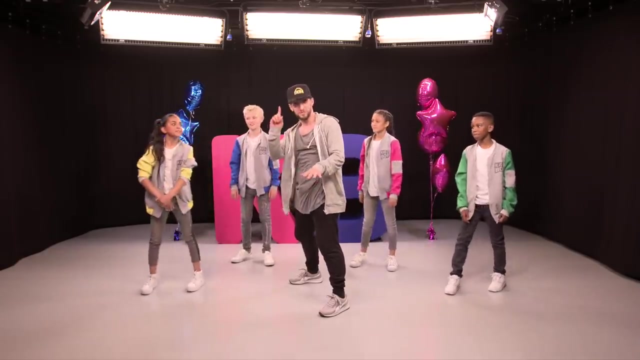 It repeats twice. you go five, six, seven. go one in two, three and four, five, six, seven. Reebok: again one and two, three and four. slide, six, finish. come on Very, very good, We are gonna go from the top, nice and slow, and then we'll try music, Okay. 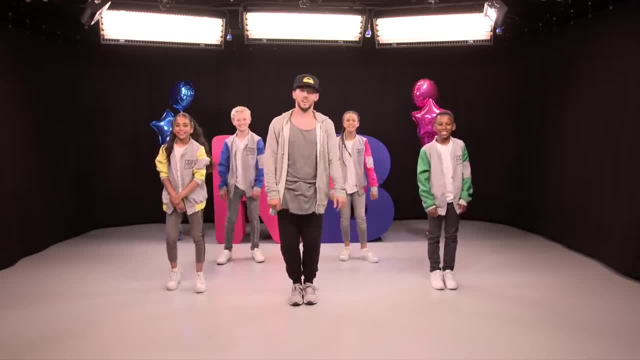 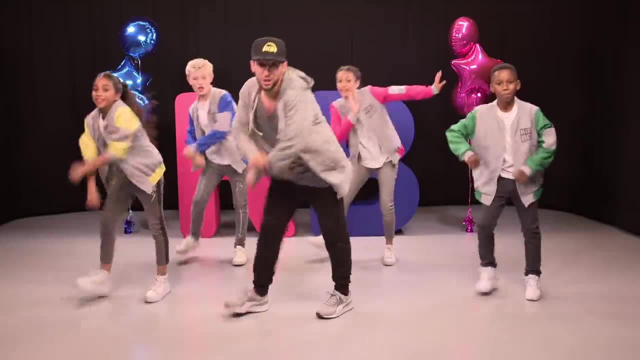 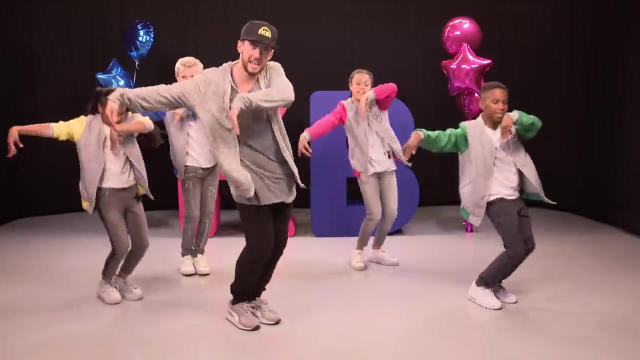 I hope you're feeling good back at home. Let's go jump nice and high ready. five, six, Seven. here we go. one and two and three and four. that's that's, that's, that's good. Good, creeping up on you So cool. That's that. that's come on, That's that, that, that, that, that, that, that, that's that's box, step, box, step.